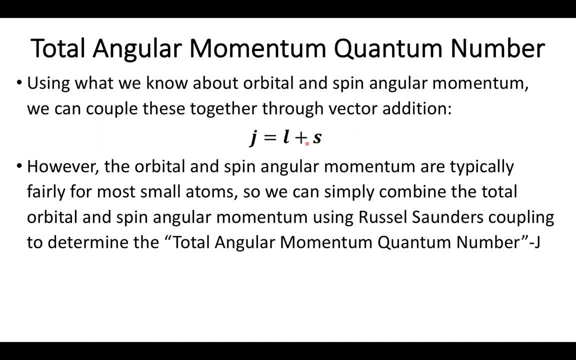 total orbital angular momentum and total spin numbers to bring together to find our total angular momentum quantum number. We're just going to call this guy J for now, because that's a little bit easier. So one of the things we have to keep in mind is, just like for the single 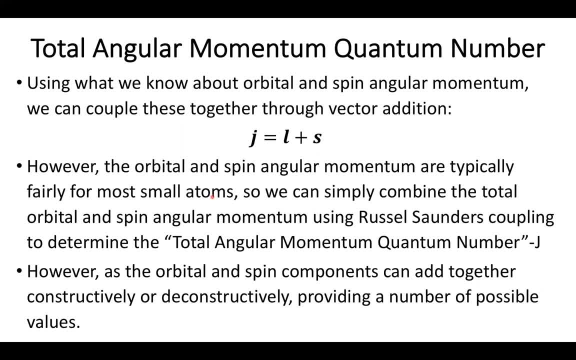 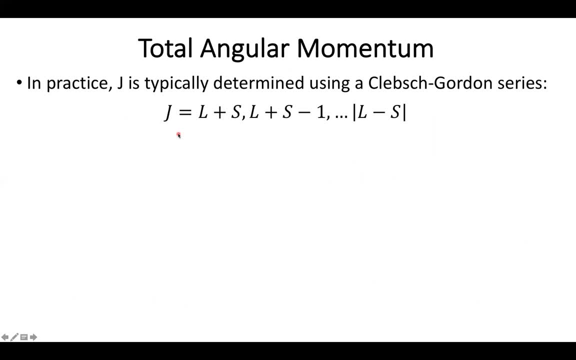 electron system. our orbital and spin components can either add together constructively or deconstructively, And this means we have a lot of possible values for J. So we can do our classic trick now of using aklepsch-Gordon series to describe the possible. 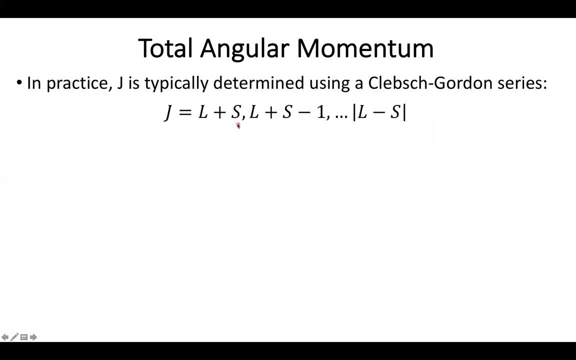 combinations, Because either our two angular momentum can be pointed in the same direction or they can be opposed, and any number of values in between, and this is where our Klepsch-Gordon series really helps shine. So we're going to have maximum values when they're aligned and a minimum value when they're. 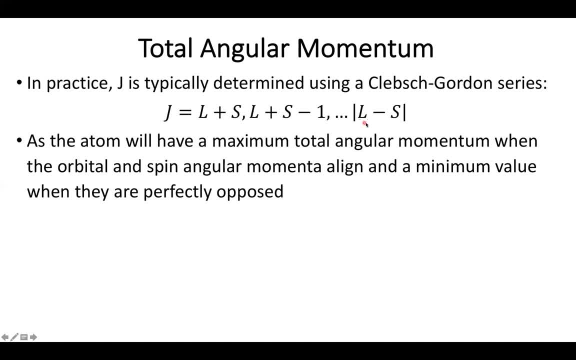 opposed and again we can't have a value less than zero, and that will become important for a couple of special cases. So most of today we're going to focus on playing around with some example systems. So if you want some practice, feel free to pause the video and work these. 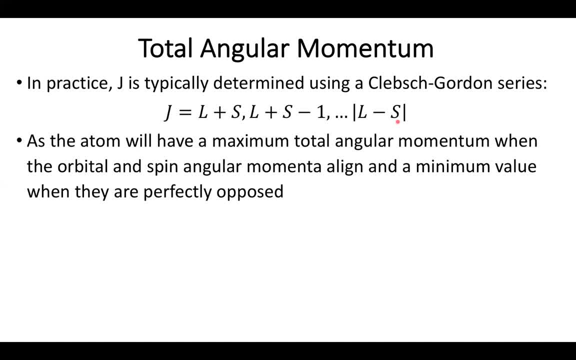 problems individually. So we're going to start with a simple system that we've looked at before and we're going to be looking at an excited state, sodium atom, where we have a single electron in the p orbital. So in this case, if I'm going to figure out my total angular momentum, I first have 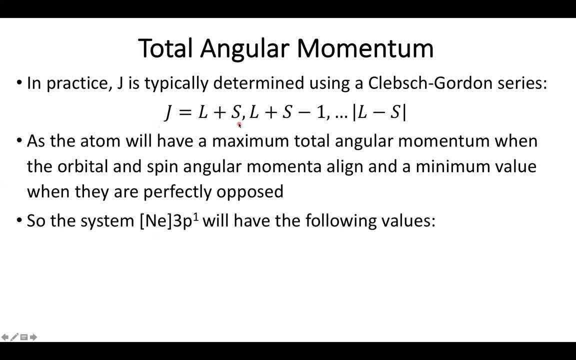 to find my orbital and spin it. So my orbital for a single p electron will always be one. There's nothing for it to align at, and again we get to ignore all of the closed subshells. So then I've got a single electron. 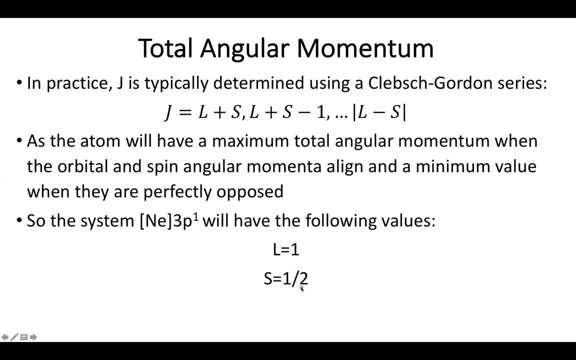 so my total spin is one half. All right, this is a pretty easy case now. So my j values say that either my total angular momentum will be aligned with a value of three or they'll be opposed at a value of one half. Yay for relatively simple systems. Now let's go ahead. 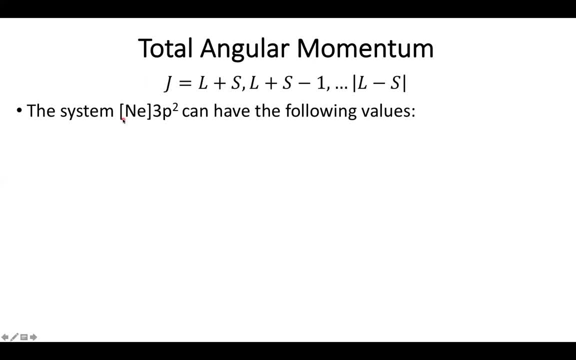 and make it a little bit more complex. Let's go ahead and look at this system for an excited state, magnesium, where I've got two electrons in the p subshell, So two p orbital electrons. So now we have to walk through what are going to be the possible values for l, s and j. 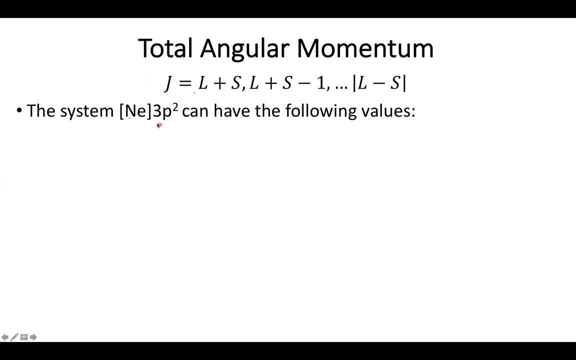 So when we do this, we'll find that we can have a maximum value for our orbital angular momentum of two and a maximum value for our two unpaired electrons of one. So when I do this, my total orbital angular momentum can either add together for a maximum value of three or cancel out for a minimum value of one. 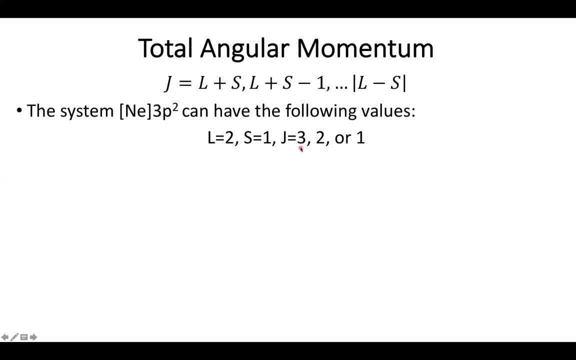 So I've got possible total numbers, But we can also have a maximum value for j and our phenomenons. that can only add up to three. So this is going to be an unpaired-al configurations, So I can also have an unpaired-al combinations. 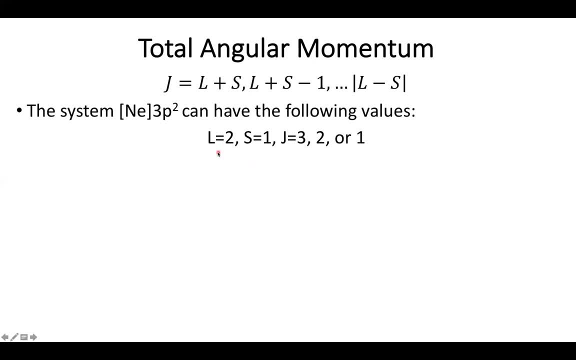 And the reason for this is that we want to have a minimum number of two that will have an angular, angular momentum. So we're going to have two unpaired-al combinations And then I'm going to have a minimum number of these two members of three, two and one. 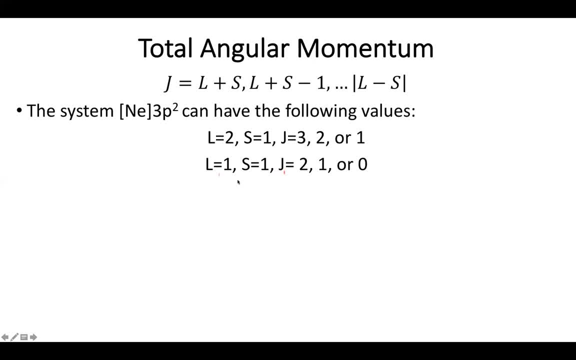 So fairly straightforward. But wait, there's more. So I can also have an orbital angular momentum of one, So this would be where my orbitals slightly cancel out. So in this case now, my j-value will have a maximum number of two, as these two angular momentum are aligned. 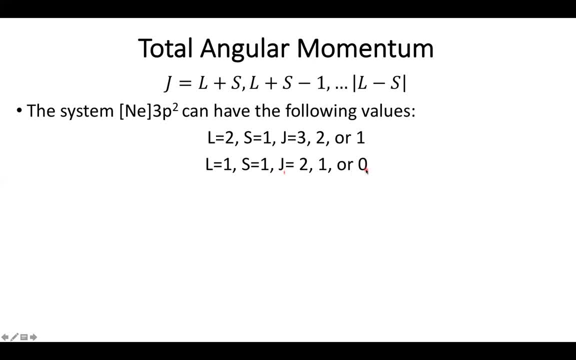 And then the minimum value of two is equal to j and there's a maximum number of j. that's not that big of a big of a difference value of zero if they're completely canceled out, which is important because if I have a J value of 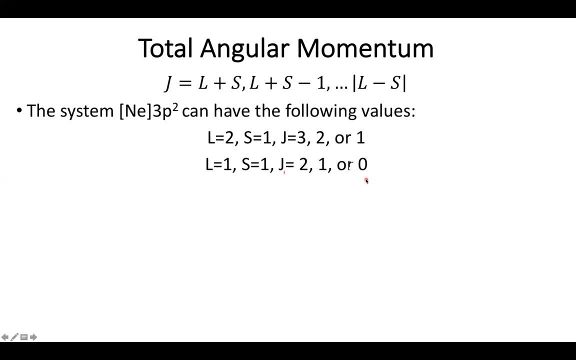 zero. this means that the atomic system as a whole we would not expect to show up in a magnetic screening. But wait, we've got yet even more. It's entirely possible that my two p orbitals can completely cancel out, So in this case I'll have a total orbital component. 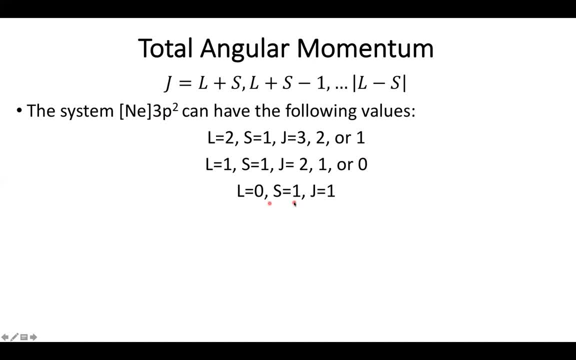 of zero, a spin component of one. Now this one gets a little bit interesting, because it turns out that L plus one is one and L minus one absolute value is one, which- congratulations, means I only have one total angular momentum value of one. Let's see how many more times I can say that. So this also makes a certain amount of sense. 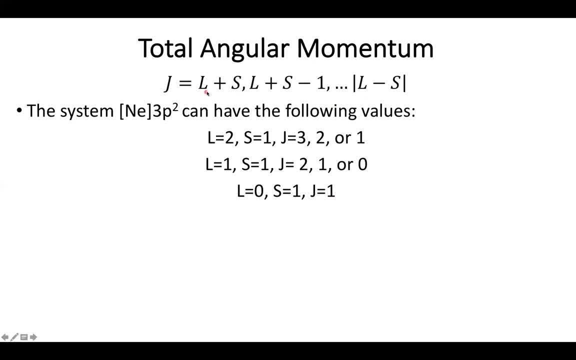 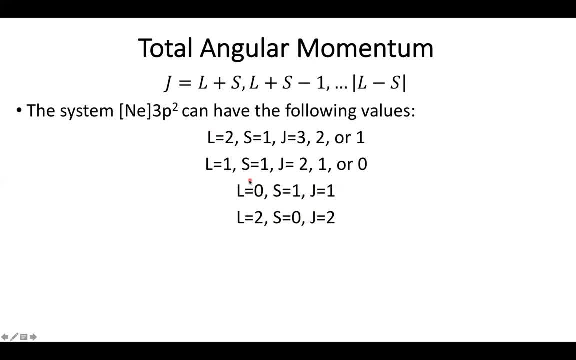 So I'm going to go ahead and do that. So I'm going to go ahead and do that. So I'm going to go ahead and do that spin number, the other one being zero. So I can have an L of two and the S of one, which 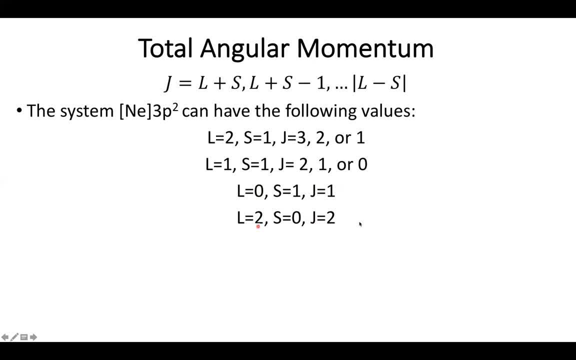 congratulations. means that my total angular momentum is the same thing as my orbital angular momentum, And this can continue for all three possible values of our orbital angular momentum, which means that- congratulations. even though I only have two electrons, this gives me a grand total of 10 possible states. Yep, this gets out of hand a little bit quickly, And even more. 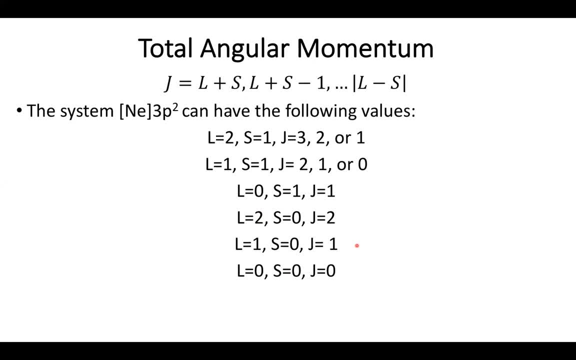 it turns out that not all of these states are accessible when we look at electron configurations. So one of the things we're going to be doing next time is we're going to want to develop a more stringent electron configuration. So we're going to want to develop a more stringent electron. 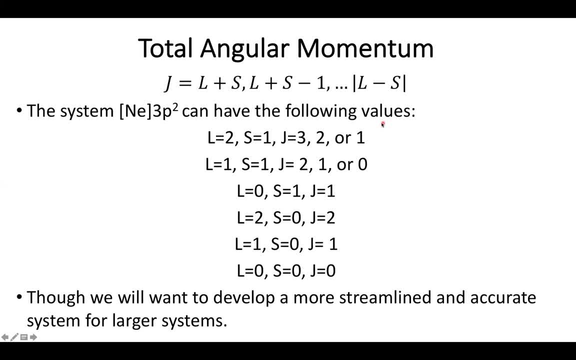 and accurate method for determining the possible states for larger systems, and hopefully one that looks at what systems are going to be actually accessible for given electronic states. So we'll continue that next time. But I want to leave you on a final note, which is that all of this assumed 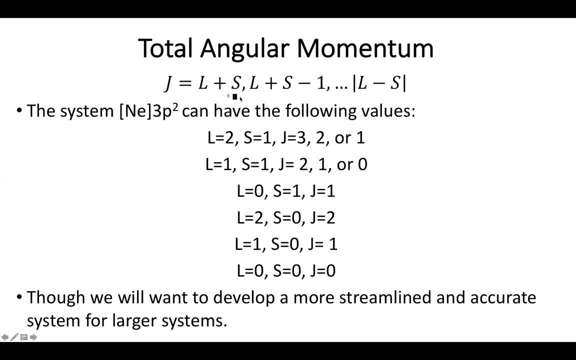 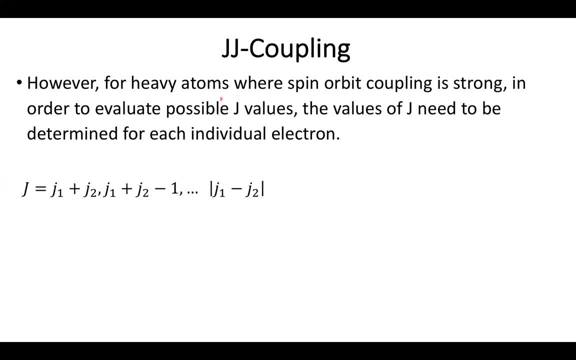 that I could be adding together my total orbital and spin components for an entire atom. This is generally pretty true for lighter atoms, but it breaks down a little bit for heavy atoms when my spin orbit coupling for individual electrons is quite strong. So in order to 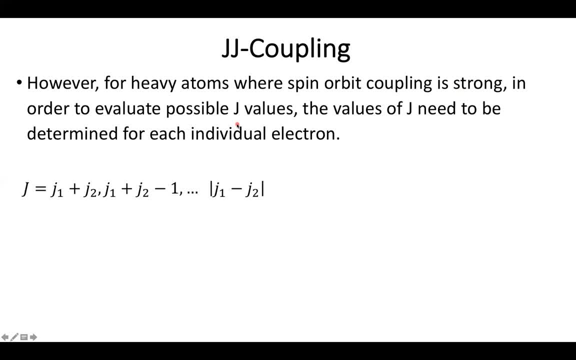 evaluate my possible total angular momentum values. what I need to do is be able to do something called JJ coupling for individual electrons, which is more or less doing again another Klebsch-Gordon series of the possible combinations for two electrons with already known J states. So this can become quite tedious, as you'll have to figure out what 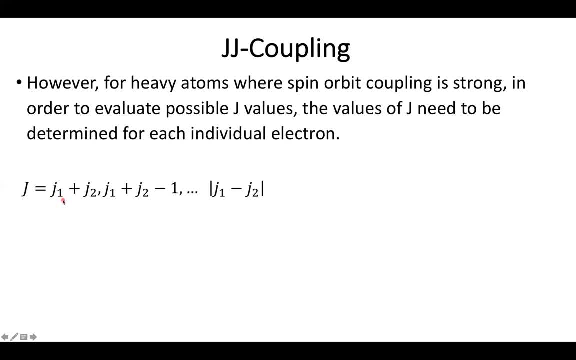 are the possible J values for any given electron and then couple it with the J values for another set of electrons and then make a series. Thankfully, it turns out that this is only really needed for relatively heavy atoms, And if I'm focused on the first three or four periods, 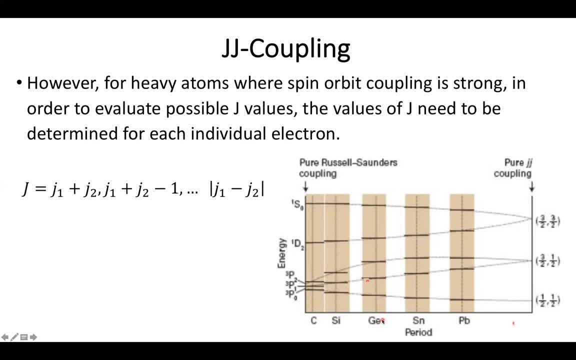 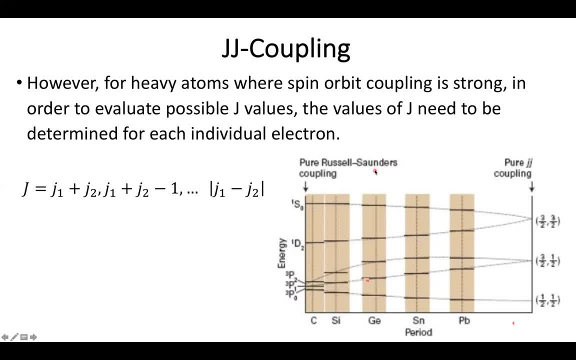 it turns out that Russell-Saunders- so this idea- I can look at just my total orbital and angular components- works pretty well. So we're generally going to be using the Russell-Saunders approach. but in case you end up looking at heavier metal atoms later in your career, you should know that. 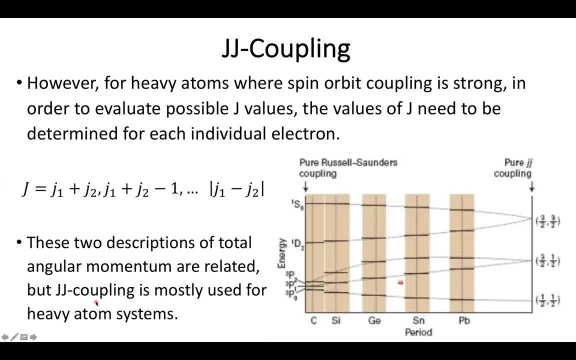 JJ coupling is something that you should take into account. So, with that said, that kind of of brings us to the end of today's lecture. So for next time, what we're going to be trying to do is finally explain these mysterious symbols that we've been using for a while, And by doing 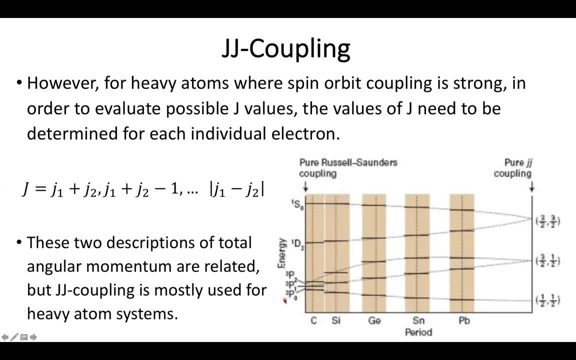 so we're going to generate a nice concise way of talking about how I can identify an individual state by its possible spin, orbital and total angular momentum values, as well as building up a better way of describing which of these states are going to be possible. 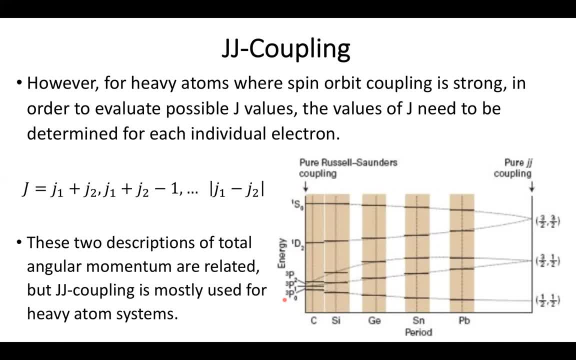 All right, thank you for sticking with me. Take care and stay healthy.